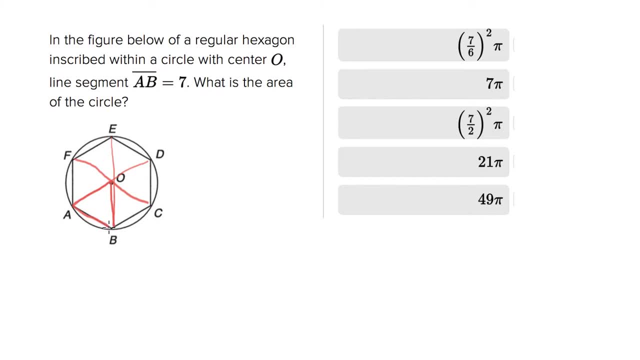 this triangle, AOB. that's an equilateral triangle And since it's equilateral, what I know is that the length of AB is equal to the length of AO, And they tell us AB is 7.. So I know that AO is 7.. AO, of course, is the radius of the circle. Once you know the 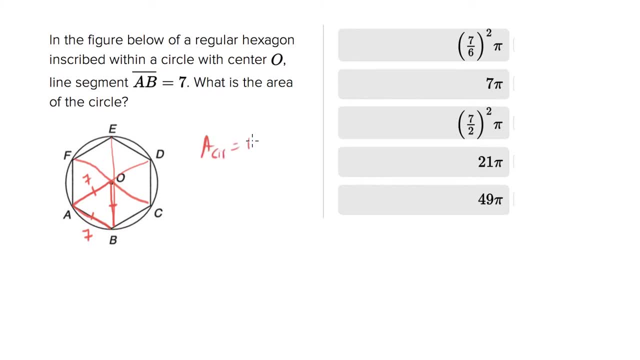 radius of a circle. you can figure out the area because the area of a circle is equal to pi times the radius of the circle squared. So that would be pi 7 squared, Or or 49 pi, which is the fifth answer choice. So if you knew that you'd be done, How could? 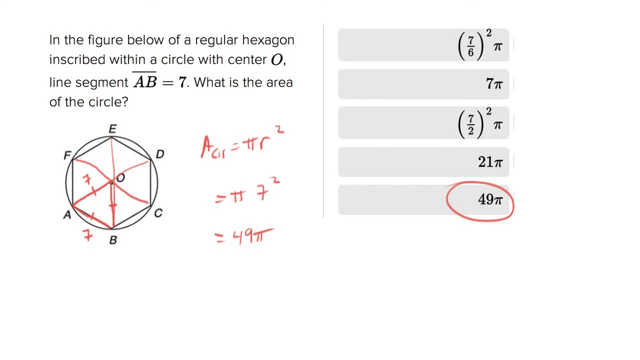 you figure that out. if you did not know that, What you would have to do is you would have to calculate the area of this, or calculate the value of this angle, And the way that you can do that, using rules that you should have memorized right. so the you know knowing. 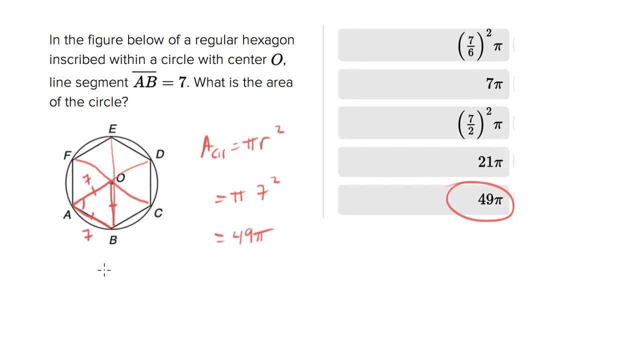 that a hexagon turns into six equilateral triangles. you may not know that, but you should have memorized the fact that the angles in a in a shape, in a regular shape, are- sorry, the angles in a in a shape. the sum of all the angles should equal the number. 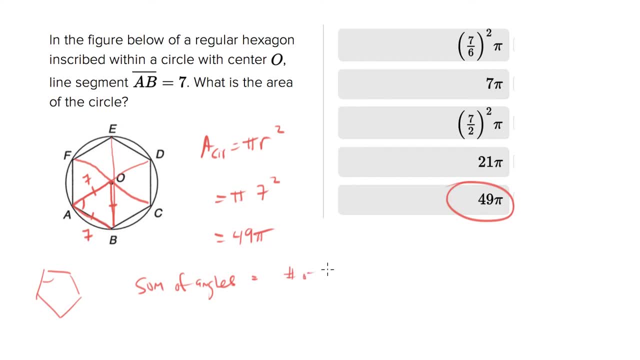 of sides, So minus 2 times 180.. That's a super weird formula, but it's one of the ones that you need to have memorized. So in this particular case we have, the number of sides is six. 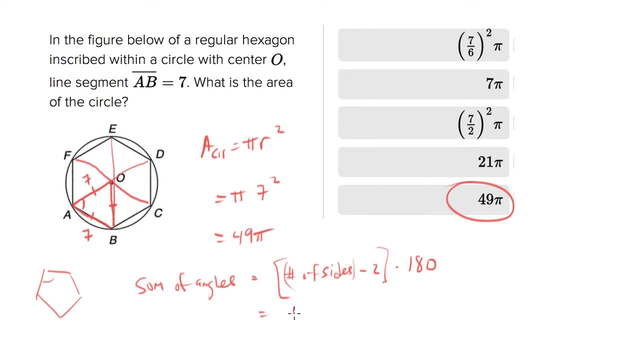 Six minus 2 is 4, so we the sum of the angles should be equal to 4 times 4 times 180.. So that is 720.. If you take 720 and you divide that by 6, which you will, you will find out. 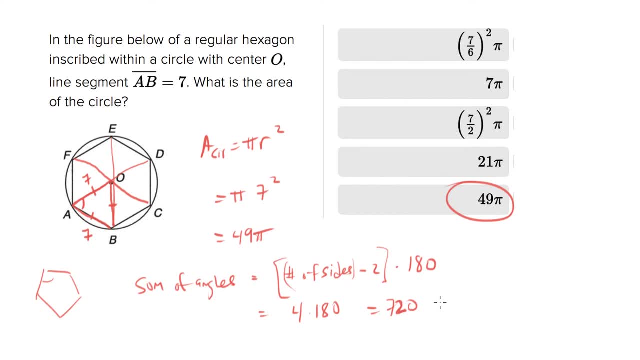 you will find. so that's the the sum of all the angles. But in a hexagon there are six angles. So if you take 720 divided by 6, what you will get is 120.. So they say it's.